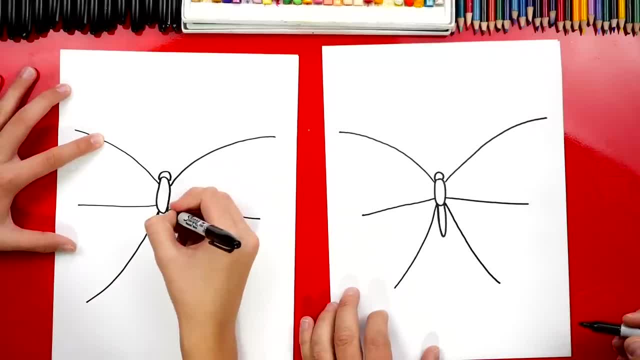 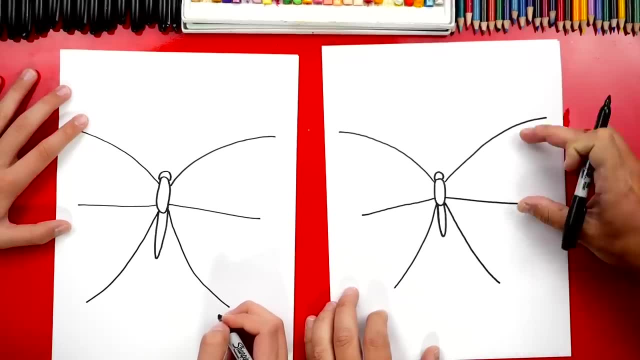 We'll draw that same curve on the other side. Now the top wing is called the forewing and the bottom wing is called the high wing. They have two wings. So now we're gonna connect these: the- the top wing, the forewing. We're gonna 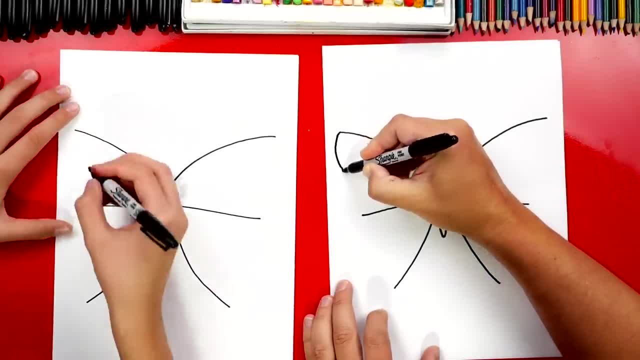 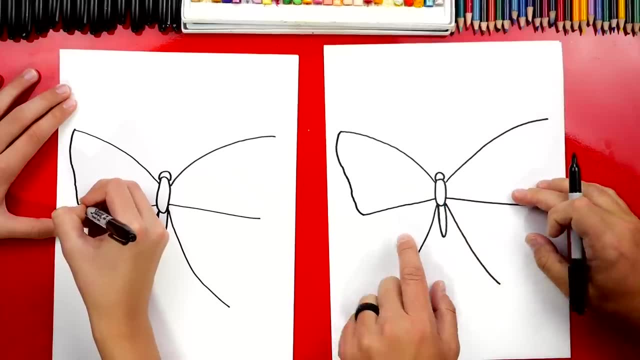 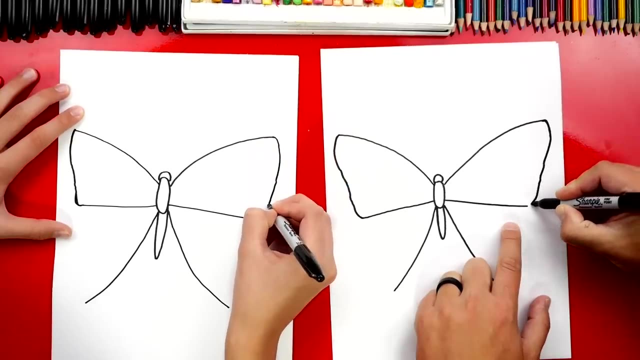 draw a curve. We're gonna start here and we're gonna curve around, and you can even put a little, a few little bumps in there, and then we're gonna come down and then curve into that middle line. and I'm gonna do the same thing over here on this side: Curve around a couple bumps and then curve. 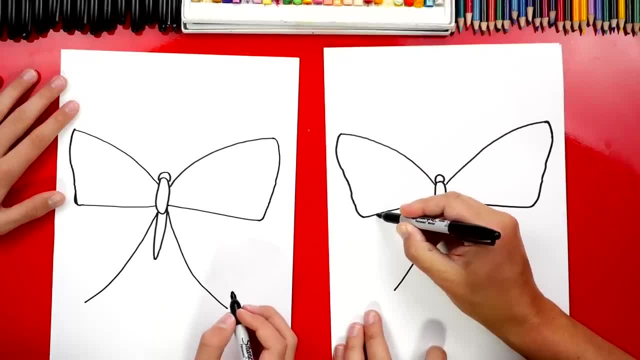 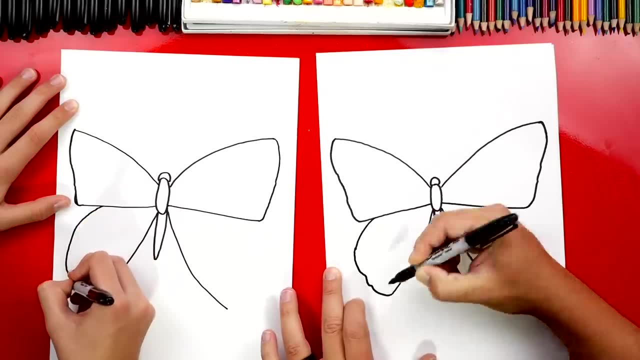 into that middle line. Now we're gonna start here on that middle line. We can come in a little further and we're gonna draw a big curve that comes out, Even a few little bumps on that one too, and then connect in. We'll do the same over here: Big curve. 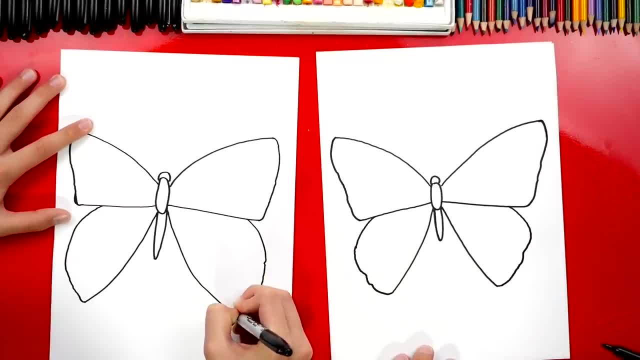 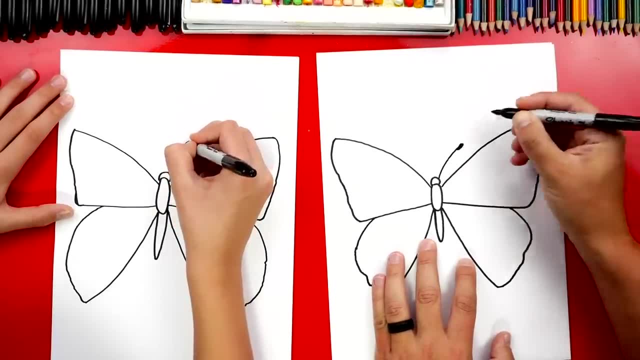 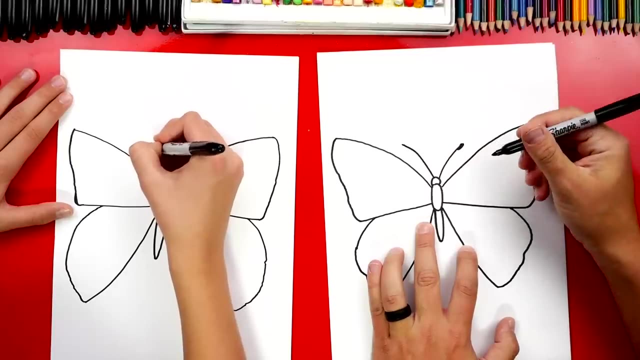 bumps and then curve in. Now we're gonna draw the antenna, We're gonna draw a little curve that comes out, but at the very end we want to draw a little club, at the end A little thicker dot. It's called a club, I think. Kind of looks like a club. Yeah, kind of. 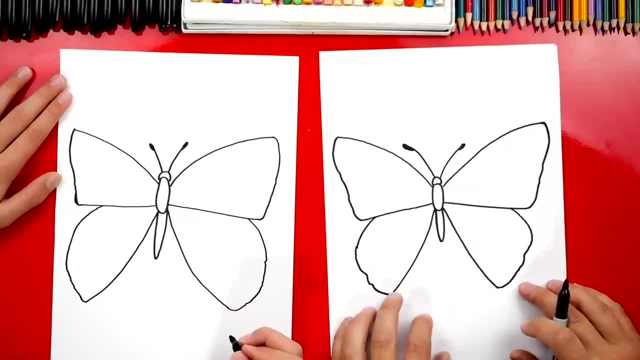 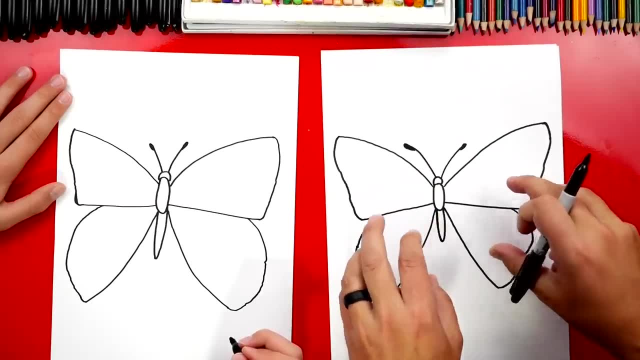 It's gonna do the same thing on the left, Left side: Thicken it up and we're gonna leave the legs off because they're underneath. We're drawing the top of our butterfly. But what's so special about monarch wings? Orange, Yeah, orange, and they have all different kinds of spots. Yeah, really cool spots. 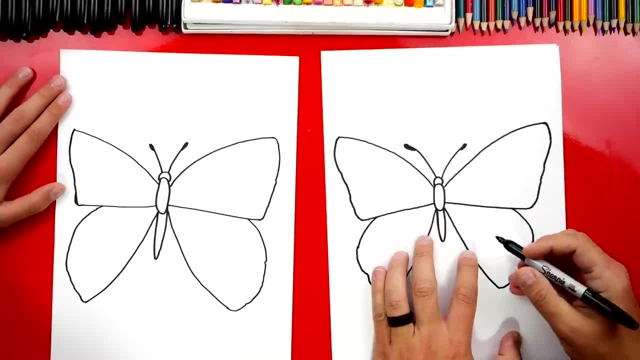 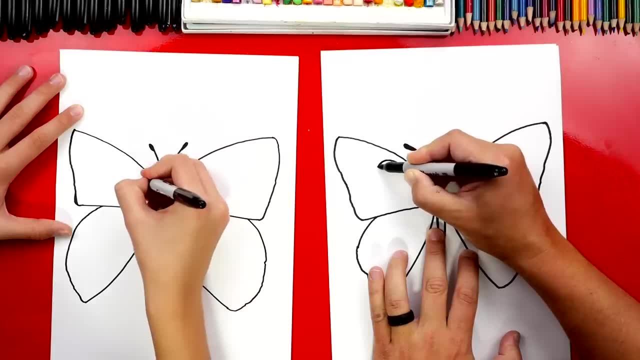 So we're gonna make all of those spots before we color it. Let's start with the four wing and we can start on the left side. We're gonna draw. this shape Comes out like this And we're gonna curve back into where we started. 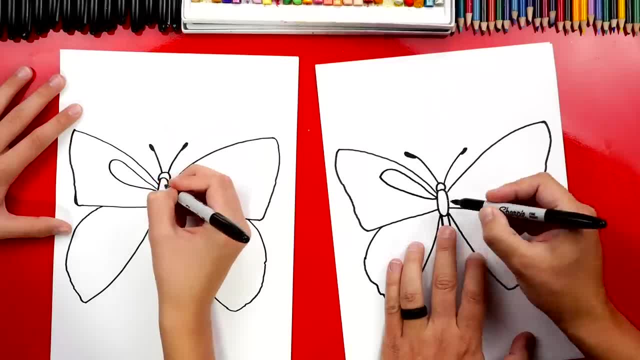 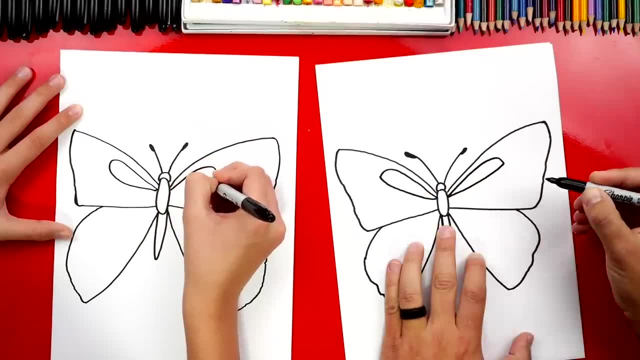 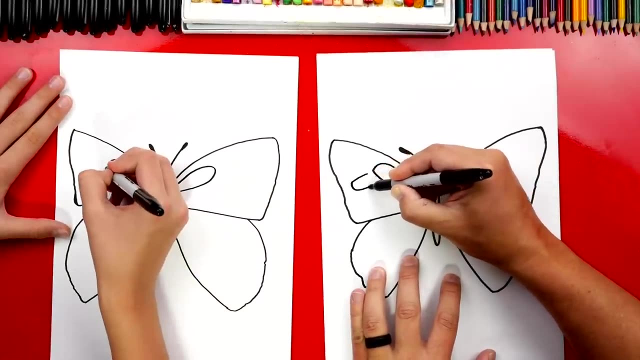 let's do the same. let's repeat all of the same steps on both wings. every time we draw something on the right side, we'll repeat that on the left side, or vice versa: if we draw it on the left, we'll also draw on the right. cool, now let's draw. we're going to draw a big shape out here, or a little. 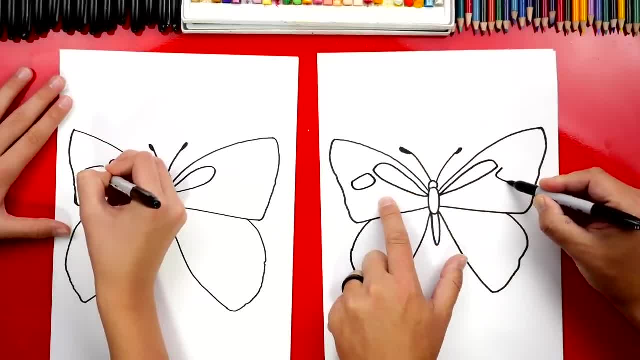 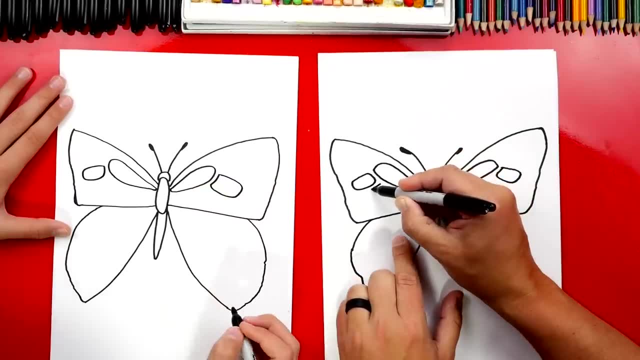 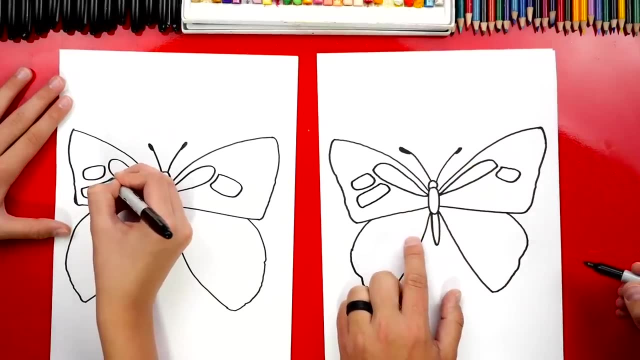 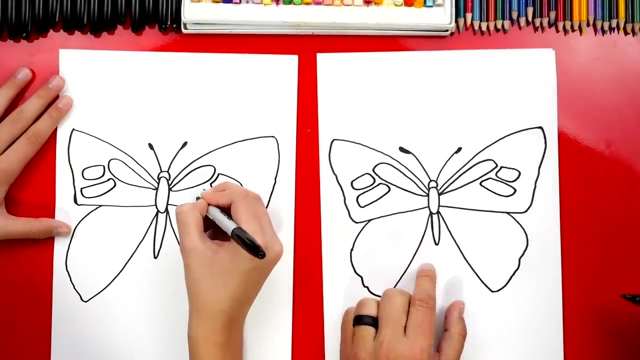 shape, actually a little oval shape. you can draw the same thing on the other side. now, the next one we're going to draw is a little longer. we're going to come out further, come back in and curve around. same thing over here a little further, come around and then back in. right now, this bottom. 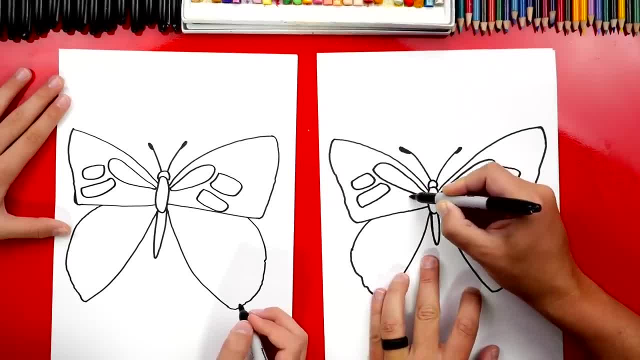 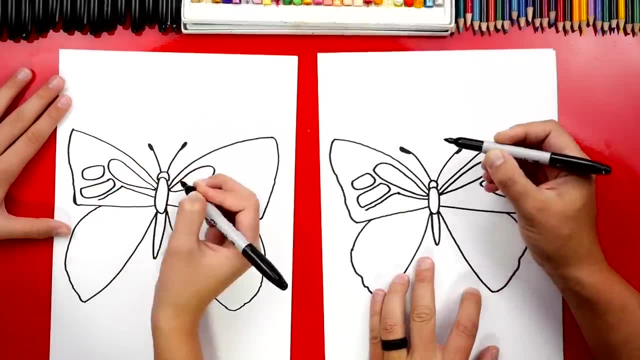 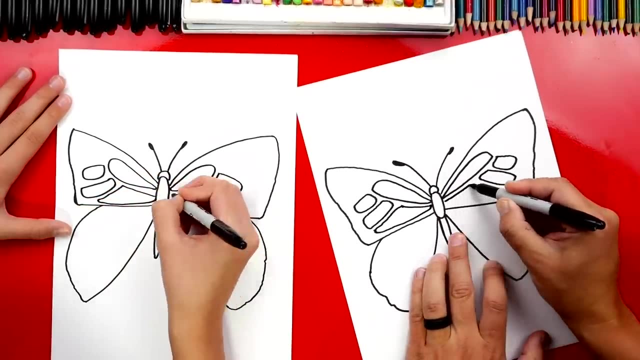 shape. right here we're going to start close to the body we're going to come out. so follow the shape, the first shape we drew. then we're going to curve and follow that third shape and now we're gonna curve back around to where we started. now let's do the same thing on the other side: follow the top shape. 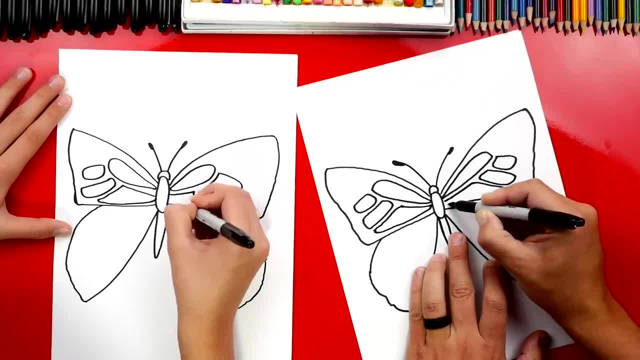 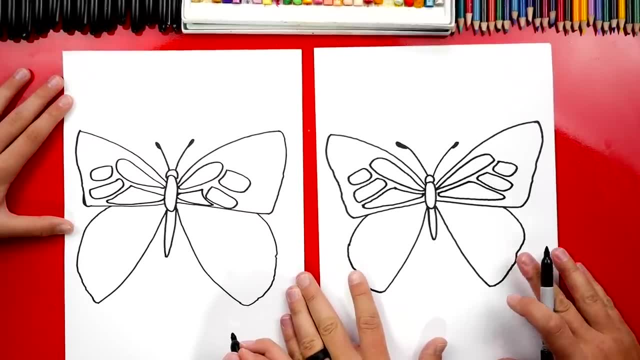 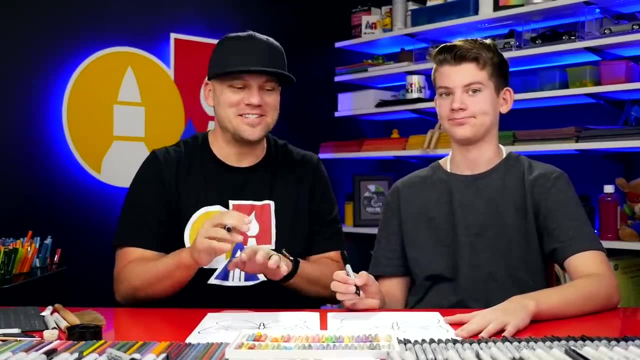 then the side one, follow the bottom of the wing and then connect back in. Jack, you're doing such a great job. now our two butterflies look a little different, right? yeah, it's okay, because the most important thing is to have fun, have fun and to practice, practice. remember. it's okay if your drawings look different. 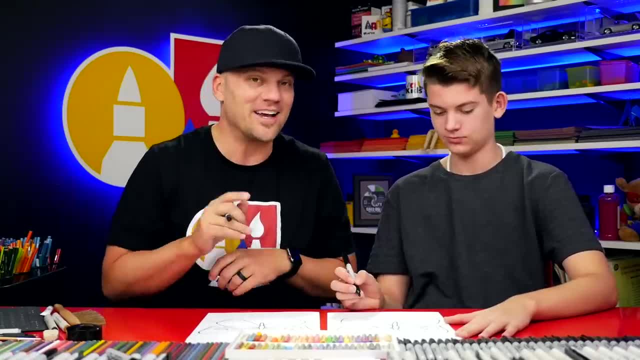 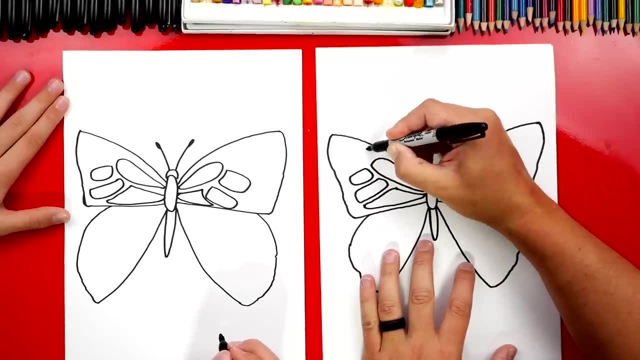 than ours. promise, the second time you draw your butterfly it'll turn out even better than the first time. yes, yeah, all right, let's keep going. now we have a few more spots we're gonna draw up here. we'll draw them all up here on the left. 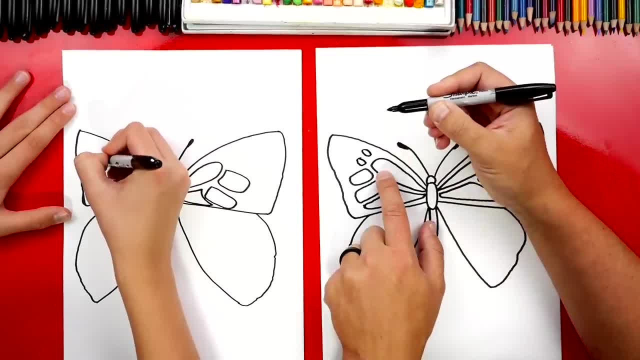 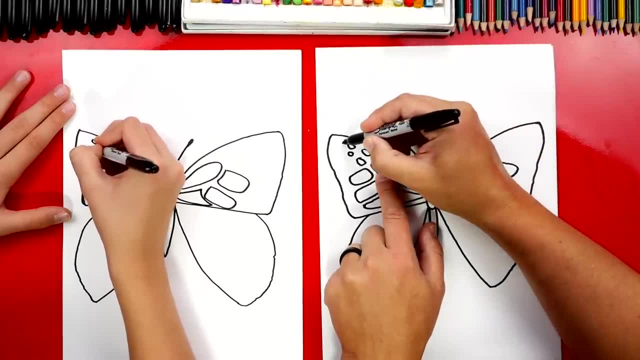 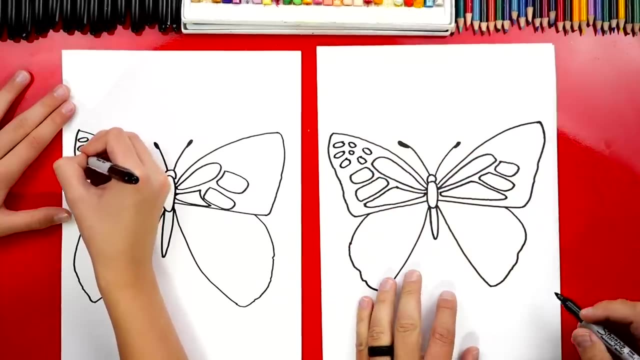 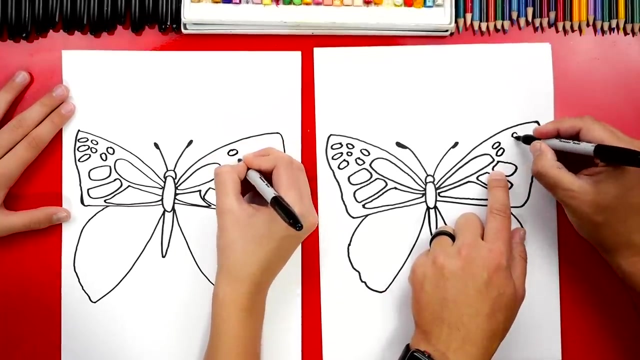 side. first I'm gonna draw two ovals, then we're gonna leave a little space, draw two more ovals- these ones can be smaller- and then I'm gonna draw three ovals that are really long on the very end. now let's do the same thing over here. we'll draw two medium-sized, two small. 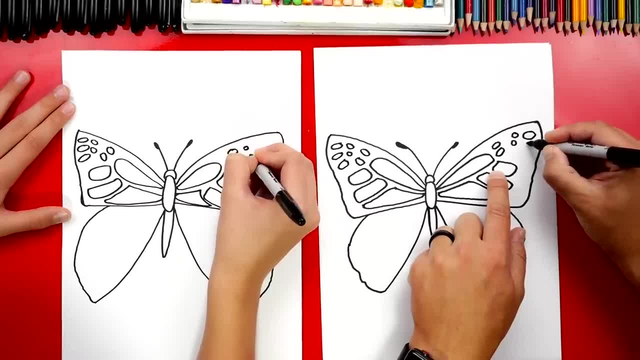 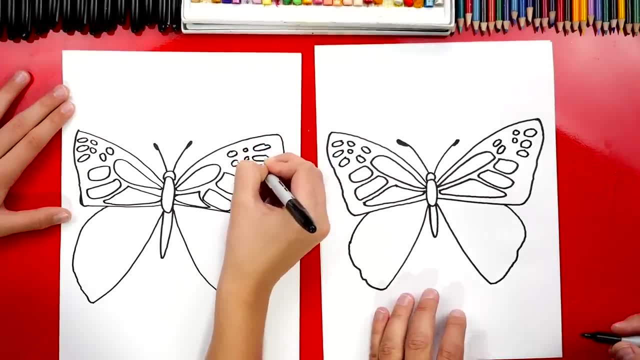 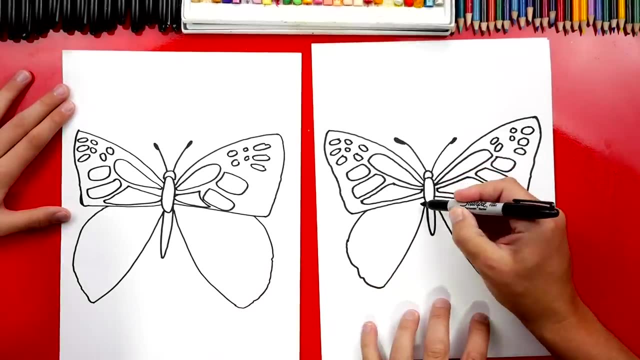 ones and then three long ones. it's really starting to look like the monarch butterfly with all the spots. now let's come down here and we'll draw the hind wings, the spots on the hind wings. we're first gonna draw a big shape right in the middle kind of looks like a raindrop shape. 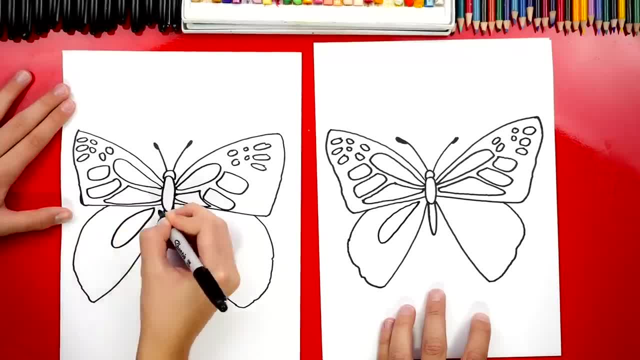 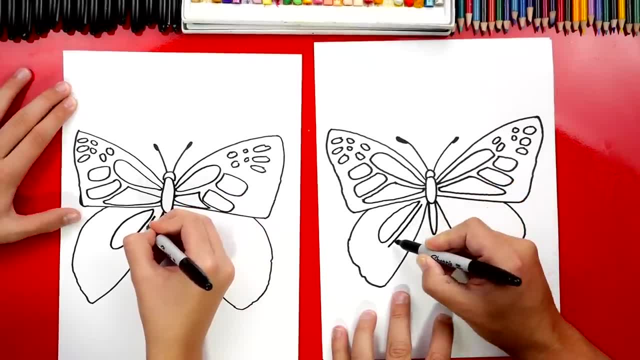 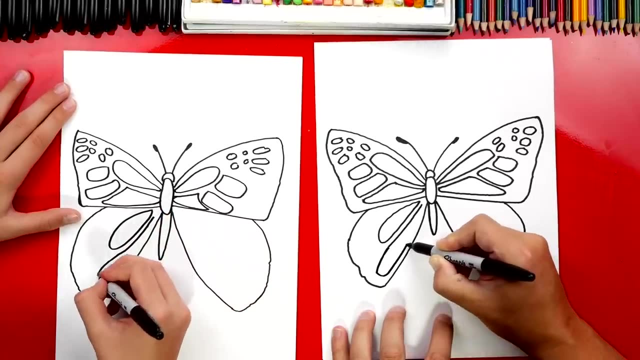 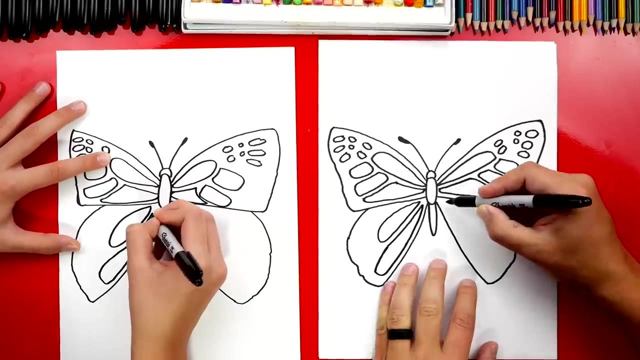 yeah, then down here at the bottom we're gonna draw a really long shape. we're gonna follow the first one we drew, go right next to it, then we're gonna come out further, then we'll curve back around and then follow the bottom shape of the wing and then connect back in. let's do the same thing over here on the right. 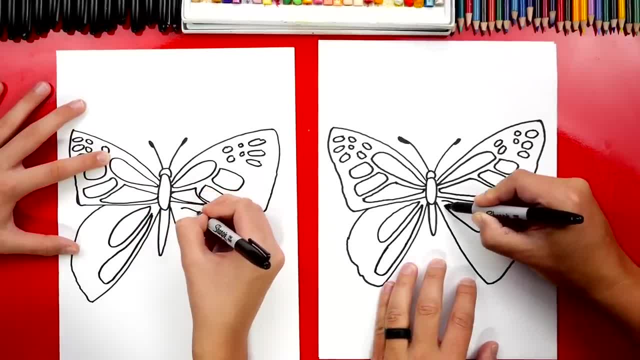 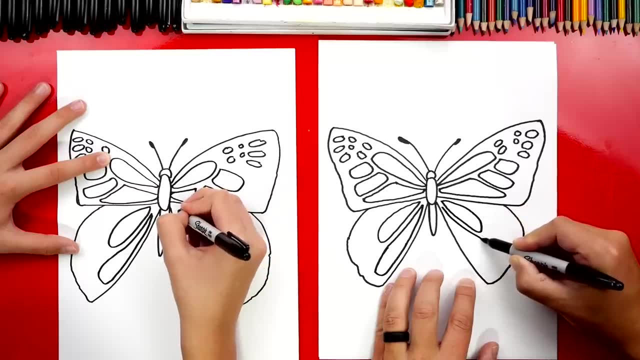 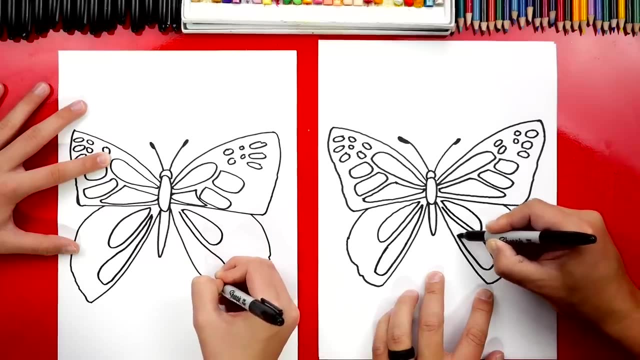 side. we'll draw that raindrop shape right in the middle of the wing and then we'll draw the fact that this is the lado shape that we drew. then we'll start close to the body, follow that first shape, then come out further to the edge of the wing, curved back around, and follow the bottom shape of the wing back. 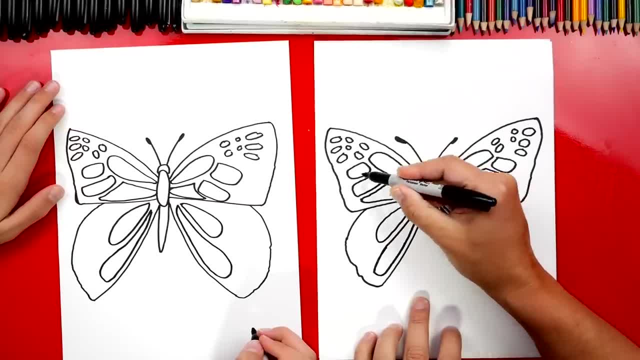 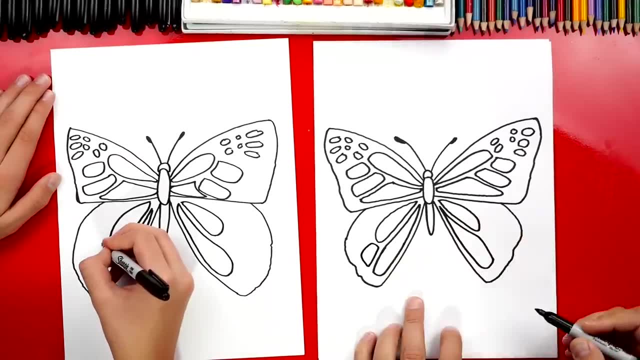 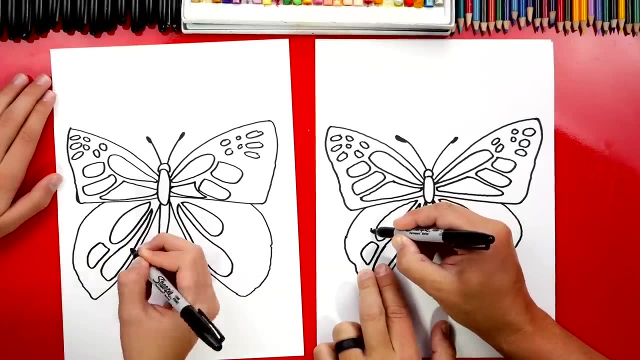 to where we started. now we're going to draw a bunch of little oval shapes, kind of like we did up here on the top wing. we're gonna start here next to the two kind of short. Then we're going to draw another one right next to that one, And 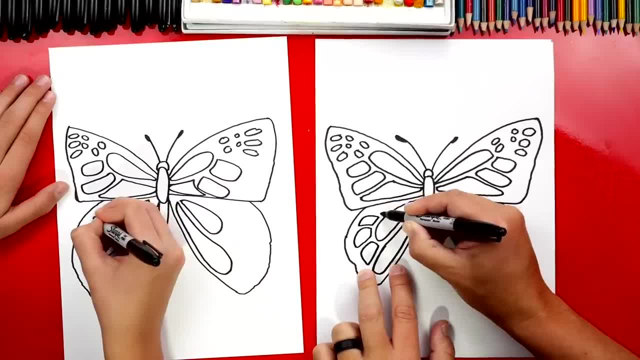 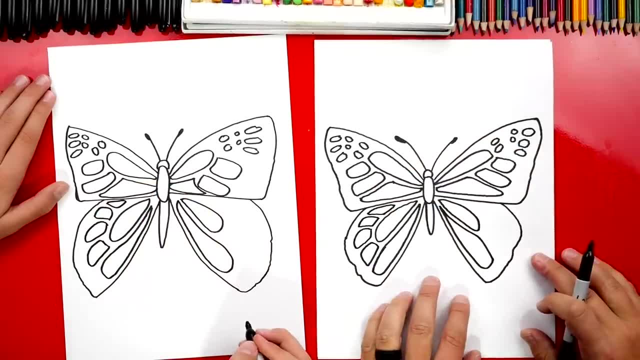 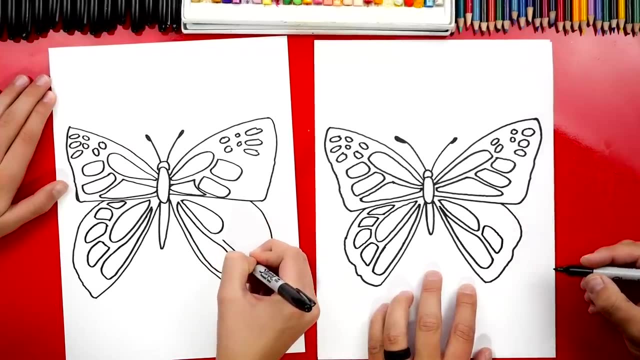 let's draw two more shapes next to those. Just fit them in right up to this top wing. Cool, That looks really awesome. Now let's do the same thing over here on the right side. We'll draw that first oval shape and we're going to draw three more. 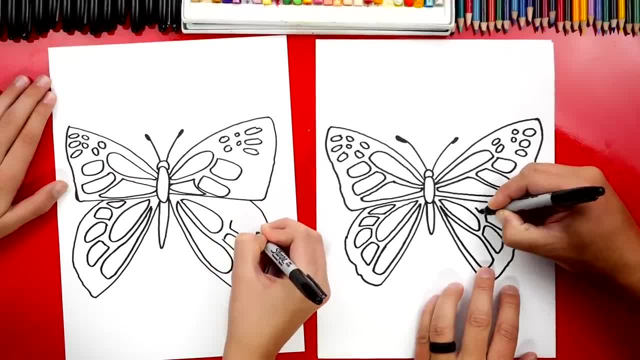 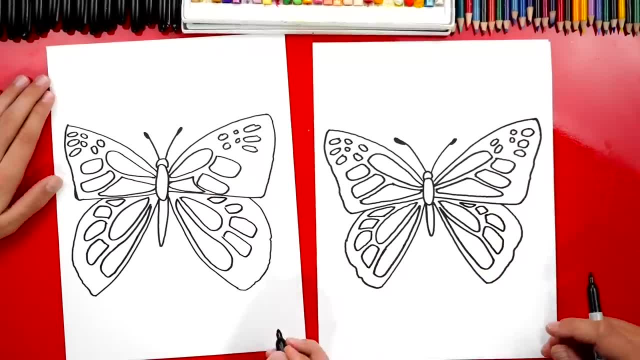 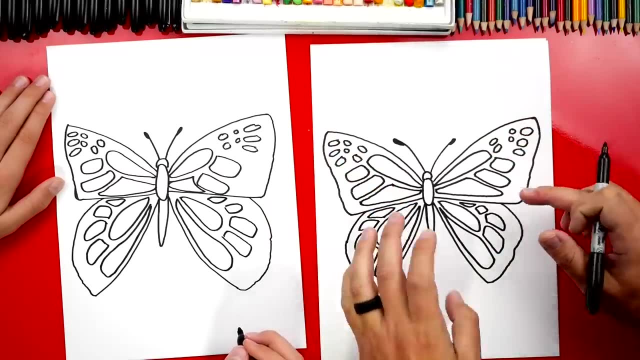 right next to that one. Well, these are a little different than the left side. That's okay. Now these are all of the orange shapes on the wing. On the very edge of each wing there's a lot of little white spots, So we're going to. 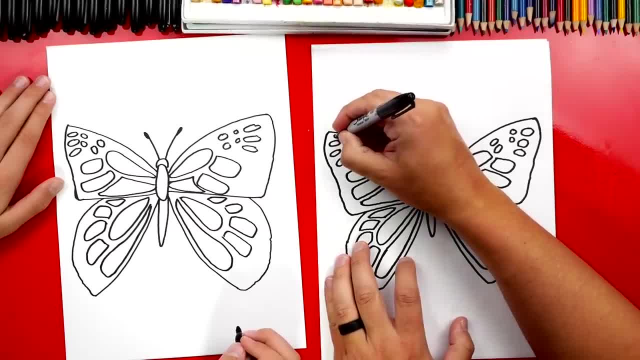 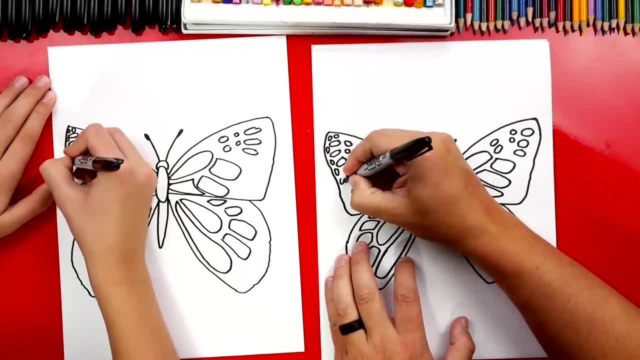 start up here on the left side and we're going to draw really small ovals and circles to fill in the edge of the wing. Now you don't have to match the same shapes or the same amount of spots that we're putting, just use your own. 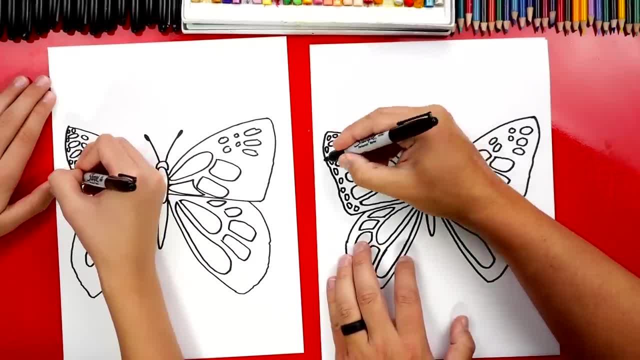 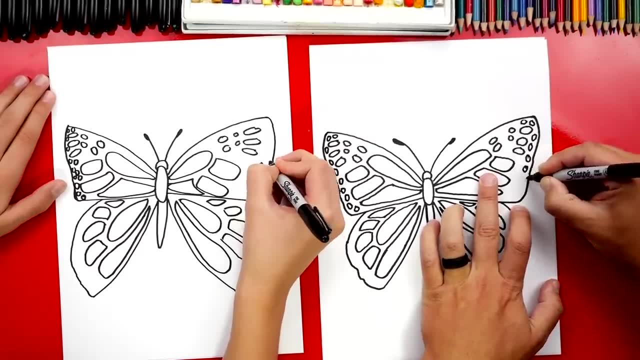 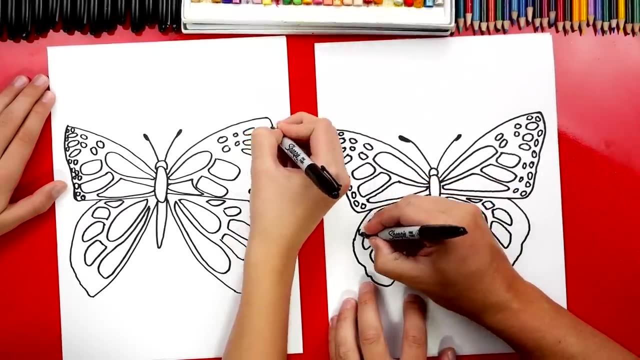 creativity and add a bunch of little white spots. These ones we're not going to color, we're just going to leave them white. when we're all done, Do the same thing over here on this side. Then we're also going to come down here and add those spots down on the hind. 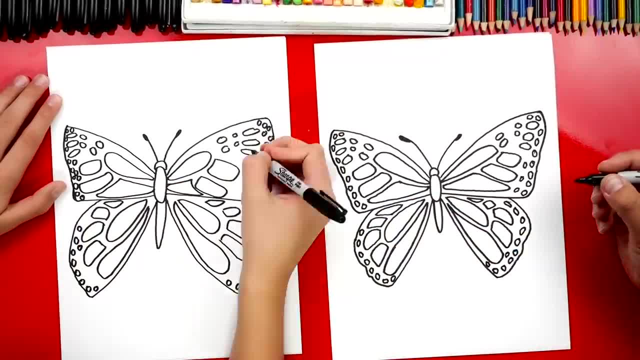 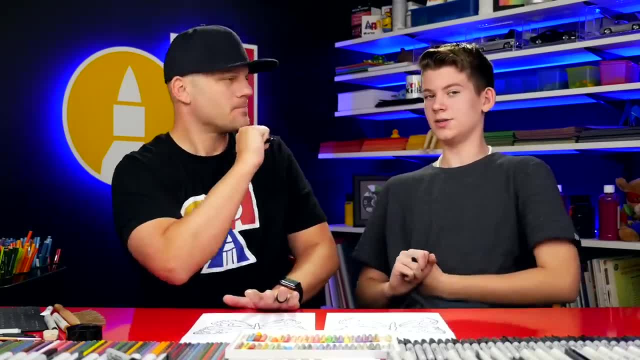 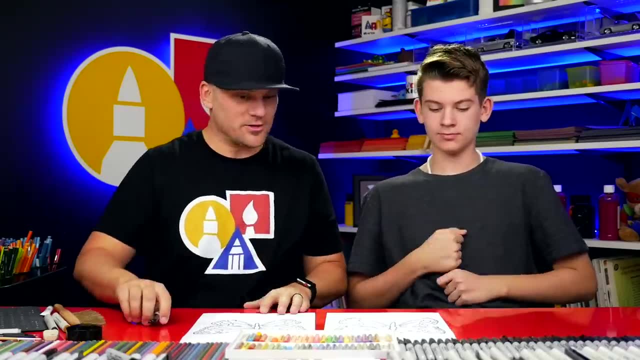 wings When we fast-forward the video or if we go too fast during a step. what can our friends do? Pause it. Yes, you can pause it. You can pause the video if you need extra time to finish a step. Now we still need to do one more thing to our